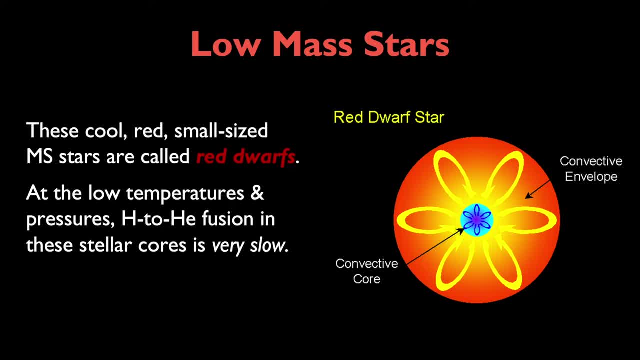 resulting in the extremely slow rate of thermonuclear fusion. Hydrogen is being fused into helium in the core, sure, but very, very slowly. These stars are also considered fully convective, meaning the only other layer within their internal structures is a convection zone directly surrounding their cores. 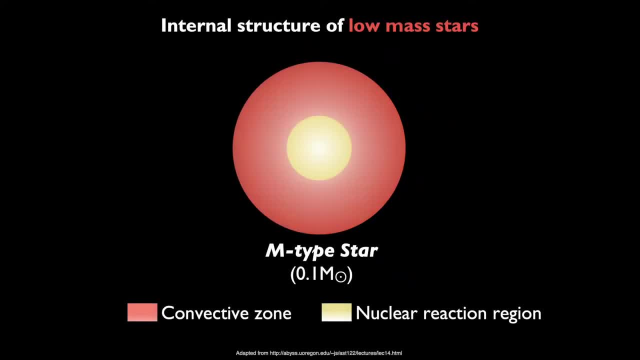 Here we can see a diagram showing exactly that for a very low-mass, low-mass star, one that's only 10% of the Sun's own mass. The inner region, the core where nuclear fusion is happening, is represented by the paler yellow circle and the convection zone just outside it. 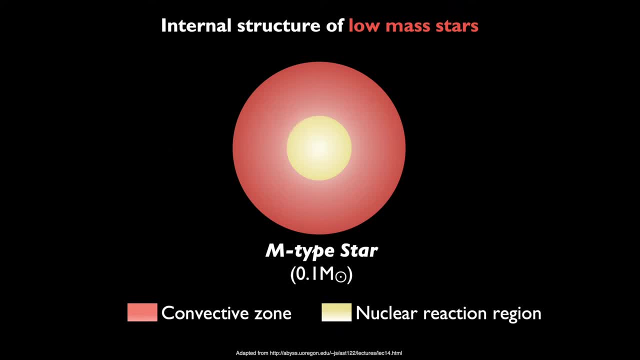 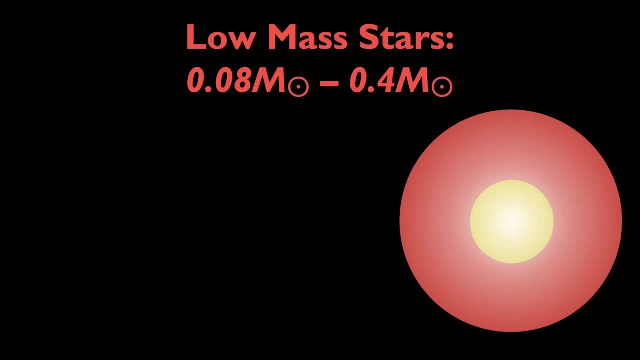 where hotter plasma rises to the surface of the star while cooler plasma material sinks inwards, is represented by the thicker red ring. Let's see what's going on inside this low-mass star, Even the lowest-mass stars that are considered main-sequence stars. 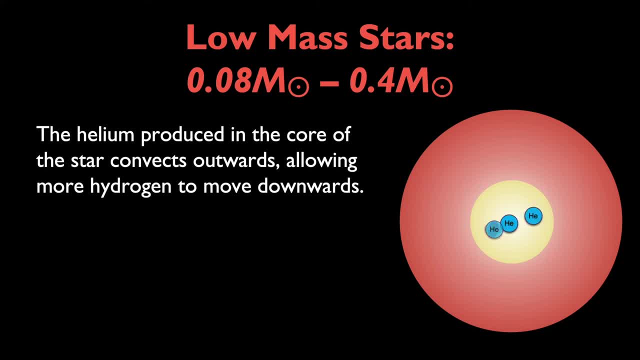 are fusing hydrogen into helium in their cores. The helium produced in the core convects outwards in these low-mass stars, allowing for more of the hydrogen in the star to fall inwards towards the core, where it too can fuse into helium. 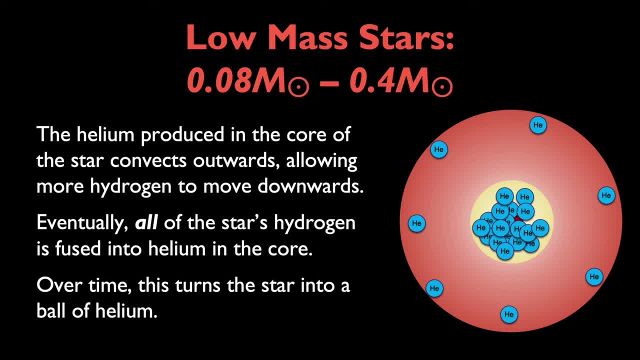 Eventually, the core will be fused into helium and the helium produced in the core will be fused into helium. Eventually, the core will be fused into helium and the helium produced in the core will be fused into helium. Ultimately, all of the hydrogen in the star is fused into helium which, over time, 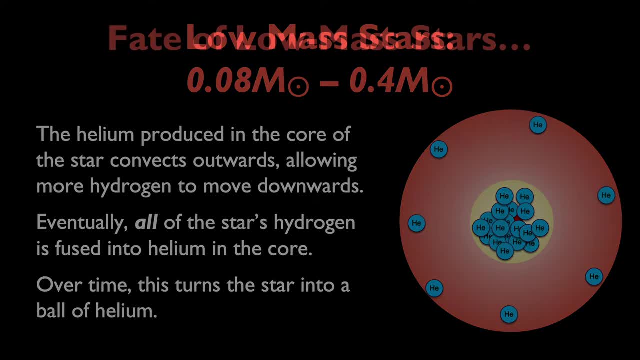 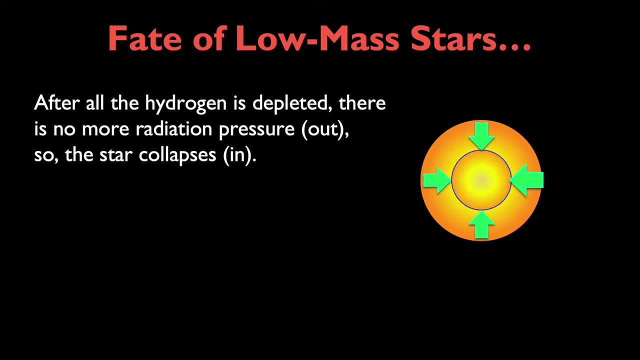 turns the star into a ball of helium as it runs out of hydrogen to fuse. Once the hydrogen is depleted, there is no more radiation pressure pushing out from the core of the star to balance against the star's weight, so the star collapses inwards. 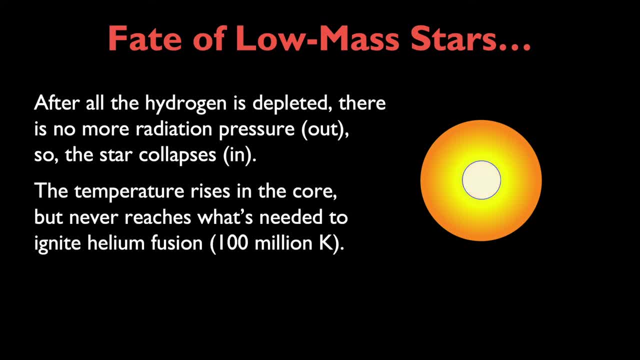 The temperature in the core rises as a result of this, but it never reaches the necessary temperature to kick-start helium fusion, which is 100 million Kelvin. Remember, the core of the star would have continued fusing the present elements into heavier and heavier elements. 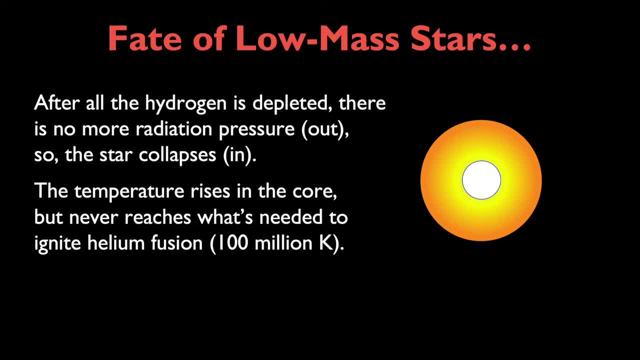 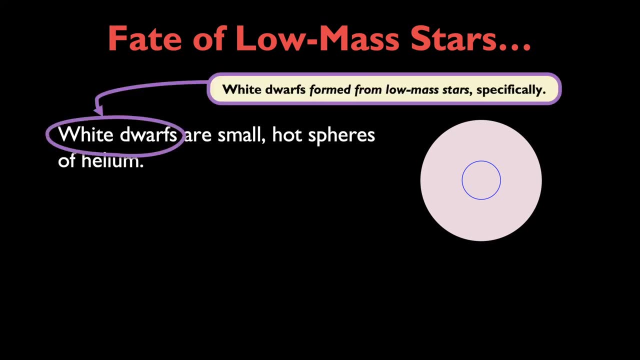 if it could, if it had the right temperature and pressure combination, but in this case it doesn't. So this remnant dead star is small and hot, and we call it a white dwarf. Now, white dwarfs, at least the ones that are formed from low-mass stars, specifically, are small.